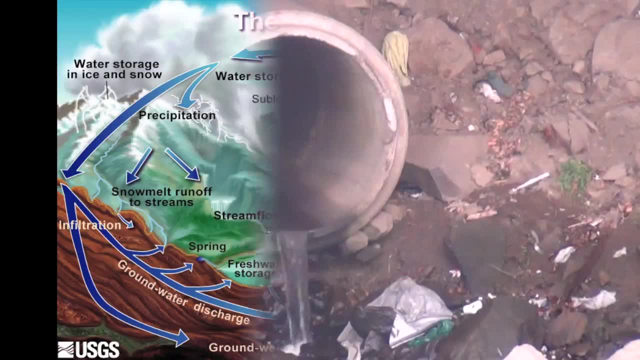 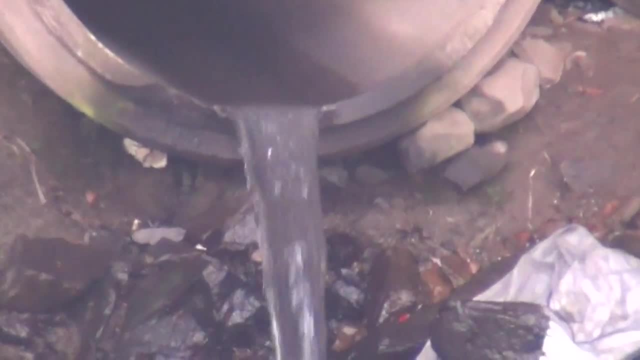 wind, water or ice. They are released from several natural and manmade sources, which we'll discuss later. Most PAHs do not dissolve easily in water, so they remain in water when they are released through industrial and municipal discharge, particularly from stormwater PAHs. 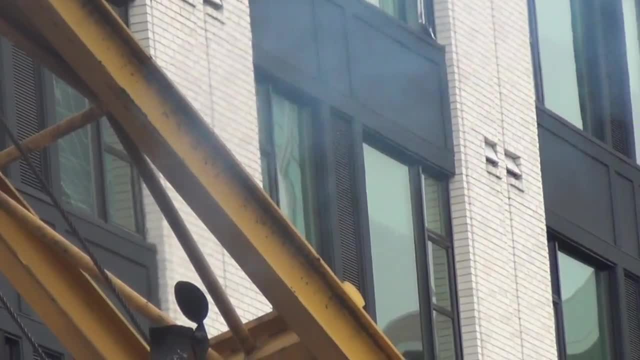 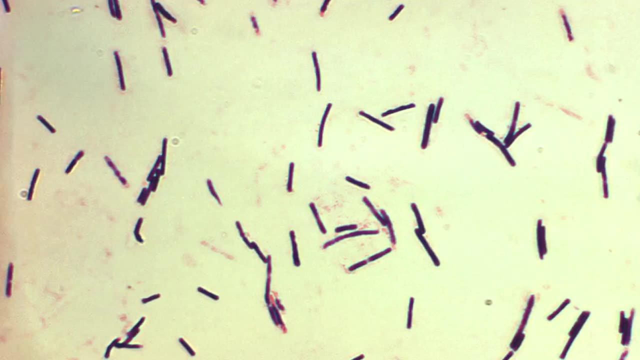 in the air can be present as either vapors or stuck to small particles. They tend to travel long distances before they drop back onto the ground. Once they are deposited into soils or water, microorganisms are the primary way in which PAHs break down in the environment. 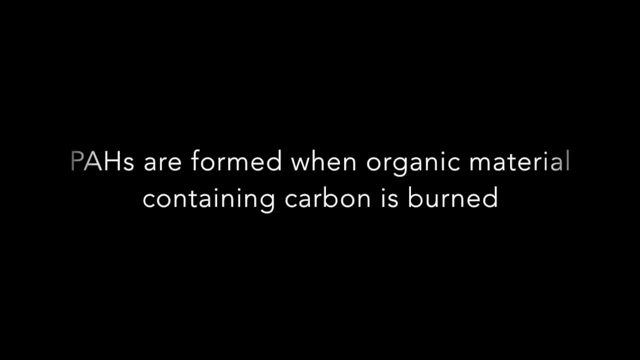 So where do PAHs come from? PAHs are formed when organic material containing carbon is burned, which means there are lots of both manmade and natural sources that can generate PAHs In the natural environment. PAHs are formed. 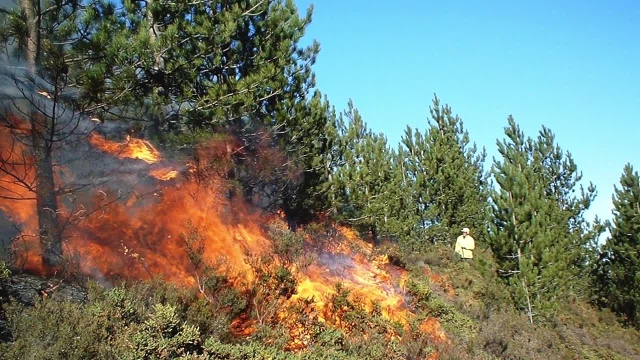 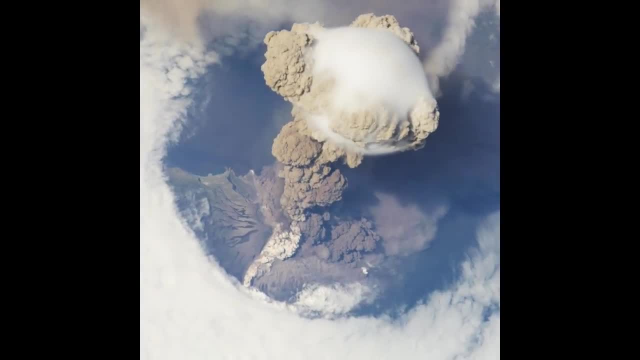 during forest and forest fire. PAHs are formed when the environment is polluted. PAHs are formed during forest and grassland fires, as well as during volcanic eruptions. PAH compounds can be found within the smoke, as well as attached to heavier particles, PAHs are also found 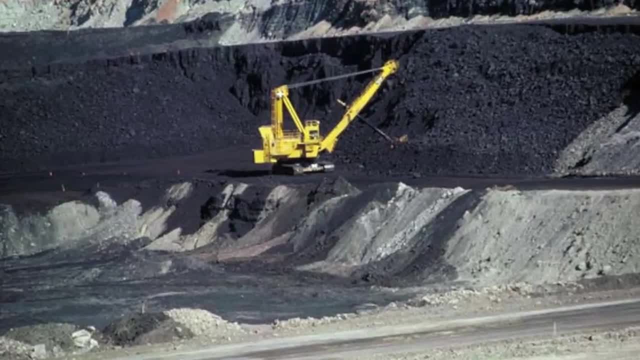 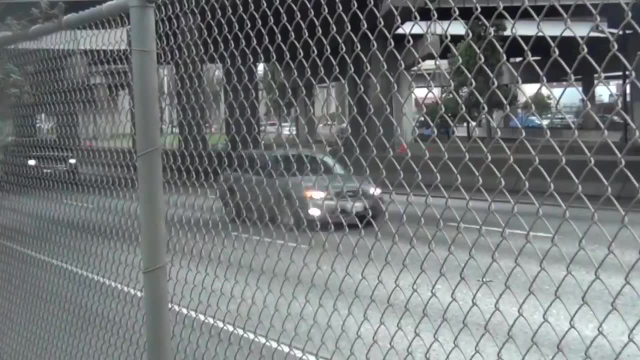 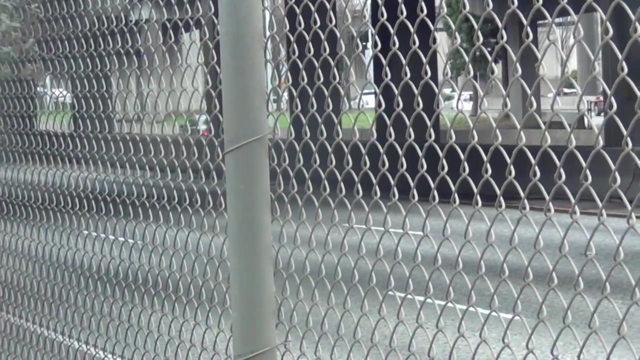 in natural deposits of crude oil and coal. Manmade sources of PAHs are also numerous. They are generated when we burn fossil fuels such as diesel during the oil refinery process, and when we burn garbage or incinerate medical and industrial waste. PAHs are also formed when we grill food, which is especially important. 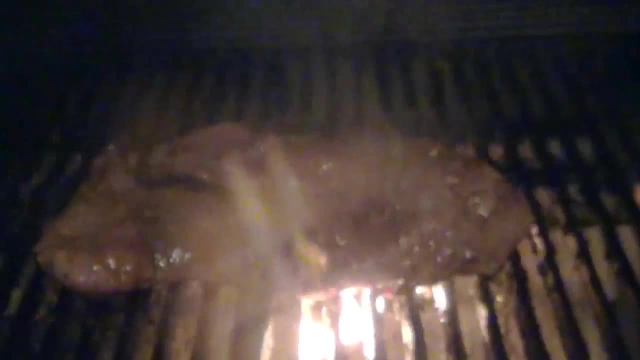 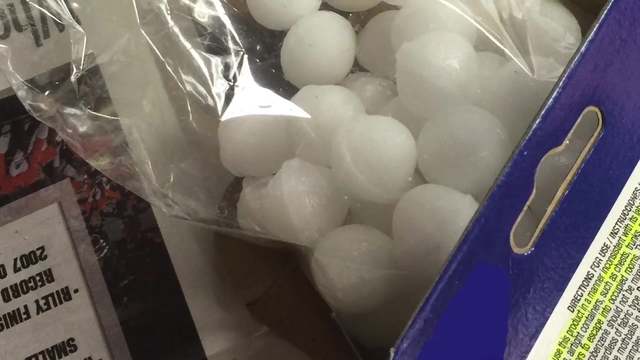 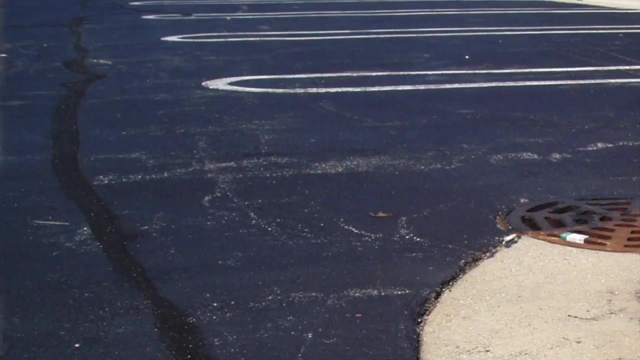 to me, since I love to grill. In these examples, PAHs are formed accidentally. However, PAHs are also used intentionally in some products as well. We use naphthalene in moth balls to repel pests and as a solvent or intermediary in many industrial applications- Coal tar. 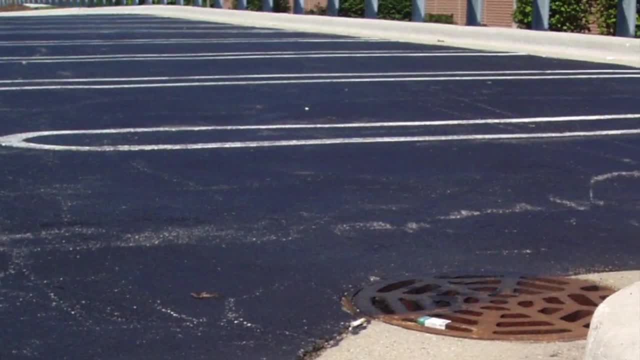 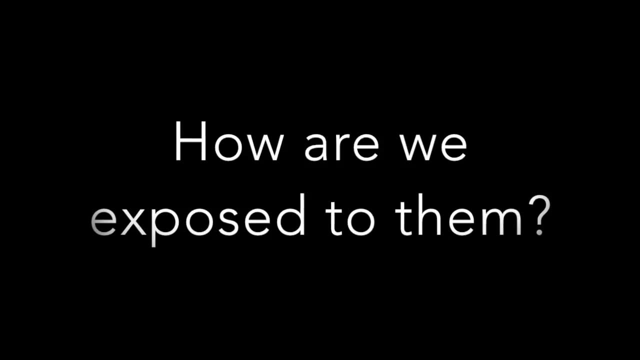 also contains PAHs and is used as a sealant for streets and parking lots, as well as in some roofing materials. Well, what about the third question? How are we exposed to PAHs? We can be exposed to something by three major ways: through ingesting it, by contact with 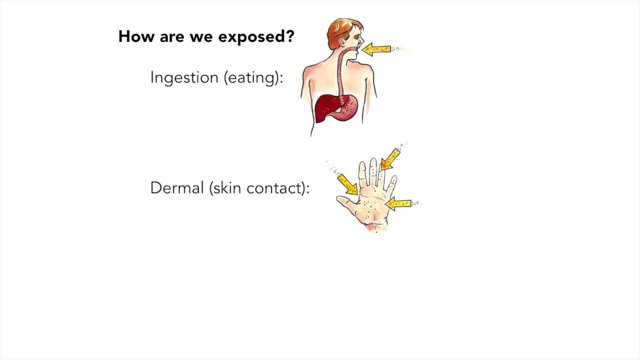 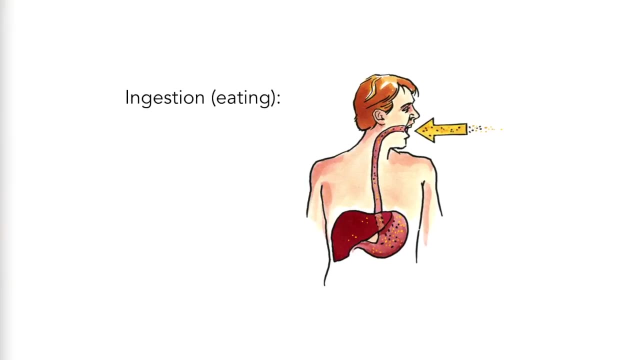 the skin or by breathing it in. For PAHs, all of these exposure sources can be relevant. One of our most significant exposure pathways for PAHs is our diet and eating foods cooked in certain ways, most notably through grilling, When food, particularly meats with high fat. 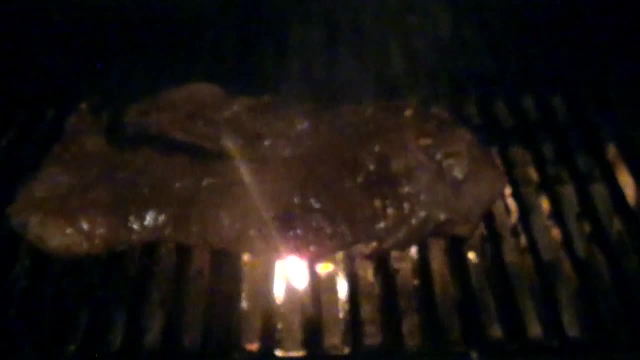 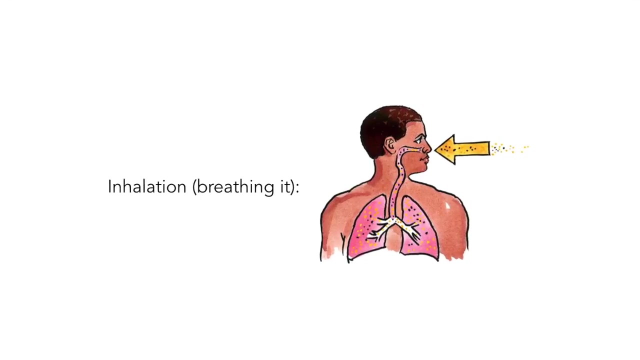 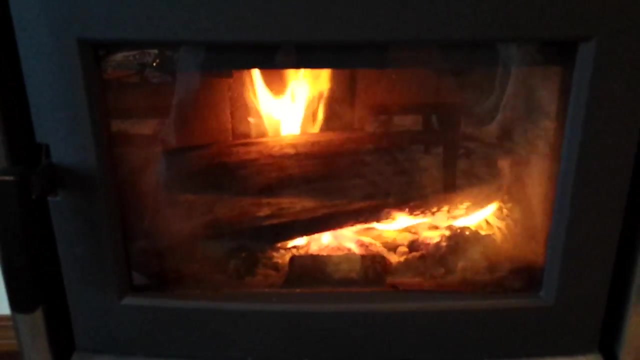 content is charred or blackened during grilling, it forms PAHs as well as other harmful compounds. Breathing in PAHs can be an issue for both the public as well as for workers. in some jobs At home. a significant source of exposure can occur through wood-fired stoves used for 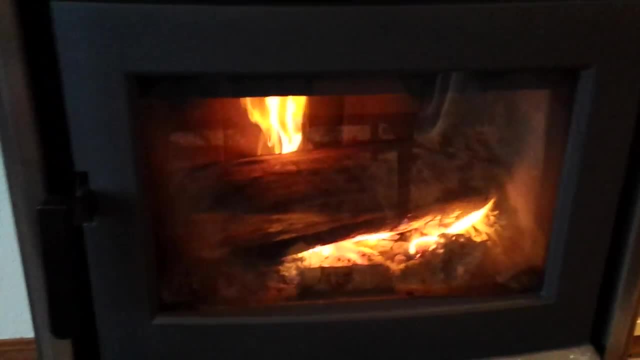 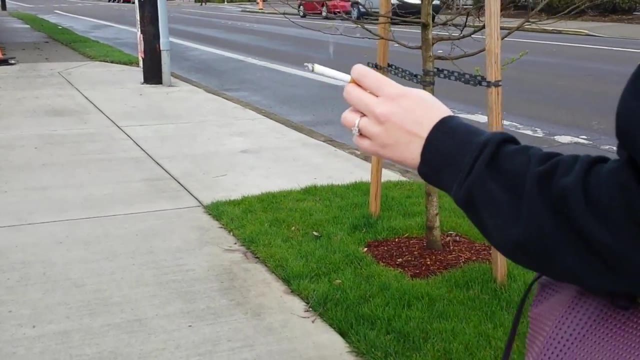 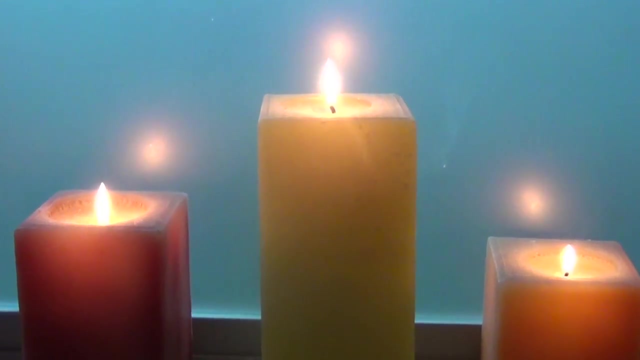 heating, particularly older stoves that are not efficient or have inadequate ventilation. Smoking creates lots of combustion byproducts, including PAHs. These not only harm smokers but others nearby, particularly kids and people with respiratory issues. Burning candles or incense also generates PAHs. 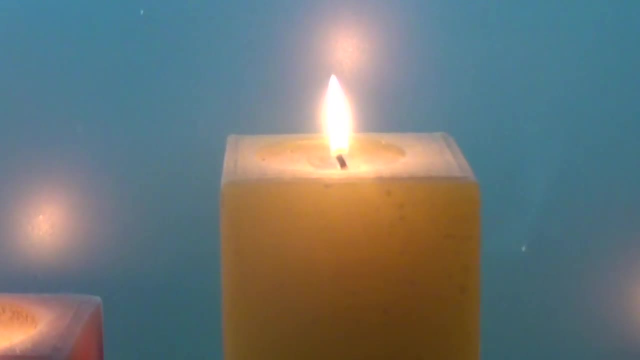 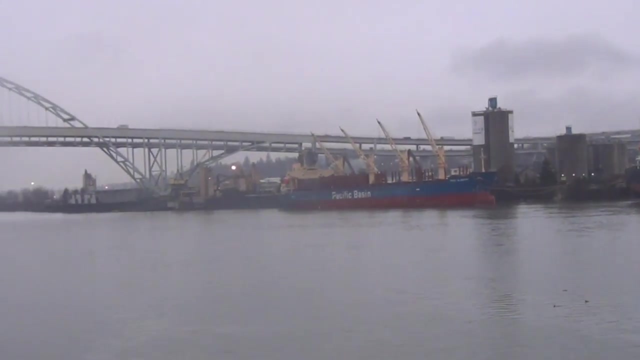 Other buildings free from indoor pollutants such as PAHs is important Outside of the home. PAHs are also found in the air we breathe, usually at low levels. Urban air generally has higher levels of PAHs compared to rural areas, particularly urban. 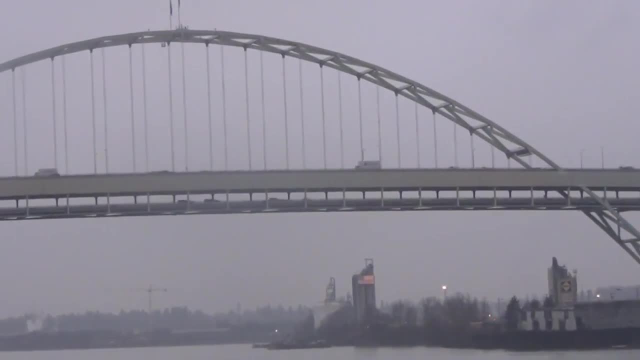 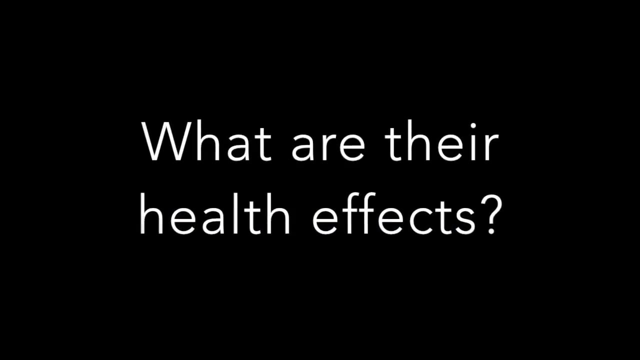 areas near construction sites, rail lines, highways and ports, since PAHs are produced by vehicles that rely on fossil fuels. Well, what are the health effects of PAHs? We have long known that PAHs can be harmful to our health. 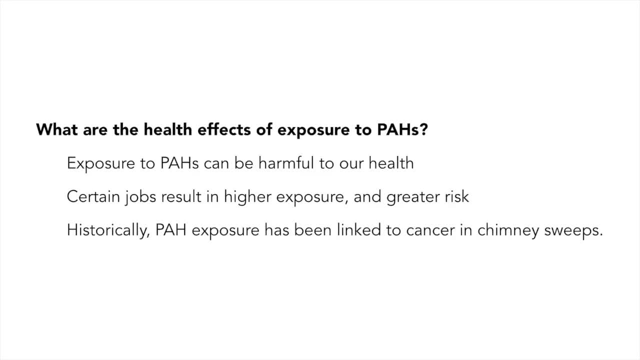 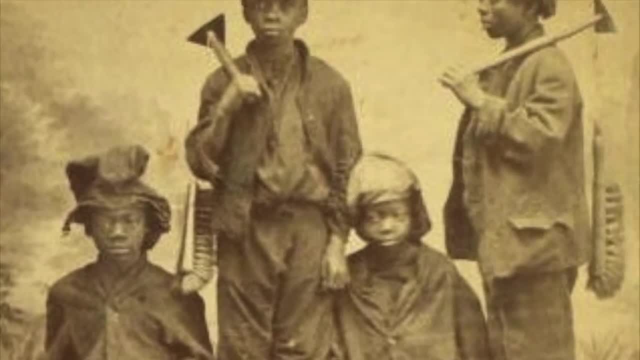 In fact, one of the first links between cancer and certain jobs involved PAHs. Back in the 1700s, young boys were employed as chimney sweeps in London. because of their small size that allowed them to fit inside the chimneys, An alert physician named Percival Pott began. 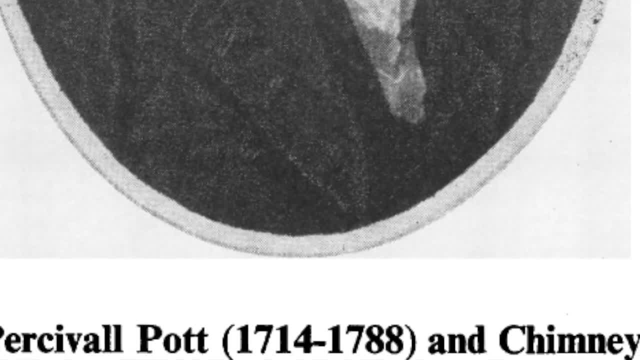 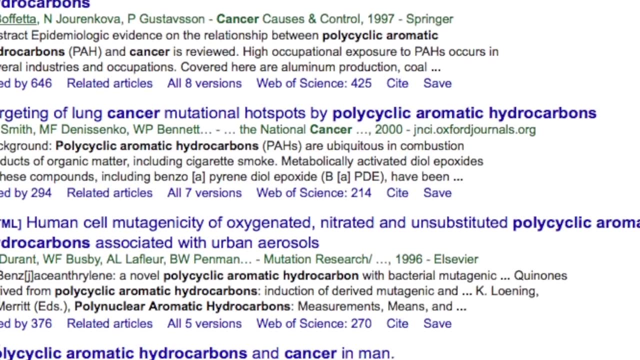 to notice that an unusual number of these boys had developed scrotal cancer, and he correctly observed that the cancers were a result of skin exposure from all the soot. We now know that the soot is full of PAHs, But what about breathing PAHs? Studies on breathing PAHs have shown that breathing PAHs 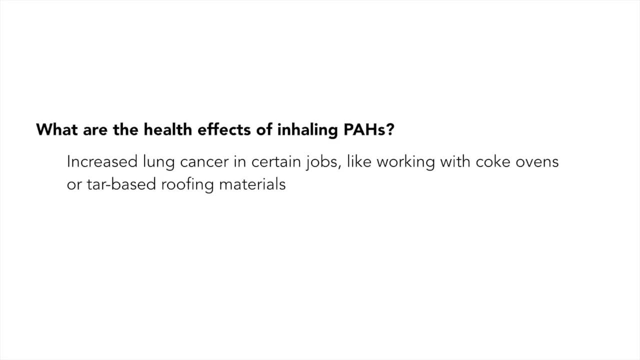 can cause lung cancer. Studies on workers have shown that increased lung cancer in certain jobs such as coke oven or roofers using cobalt-based tar materials. Cigarette smokers were also at much greater risk of developing lung cancer. Beyond cancer, many of the same inhalation exposures can result in negative effects on. 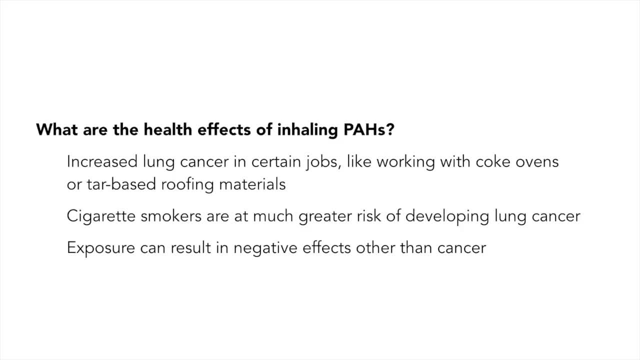 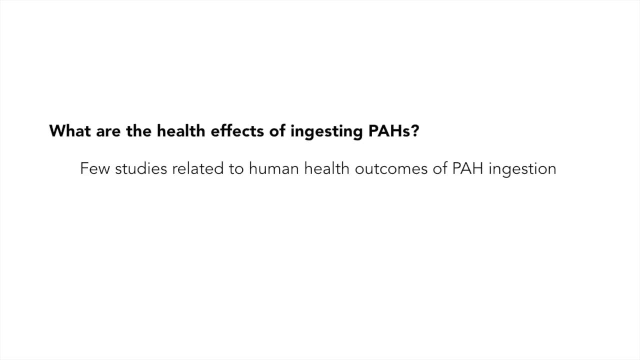 breathing, chest pain and irritation. frequency of cough and throat irritation. Ingesting PAHs is still the biggest exposure pathway for the non-smoking public. There are only a handful of studies that have shown that non-smoking PAHs can cause lung cancer. 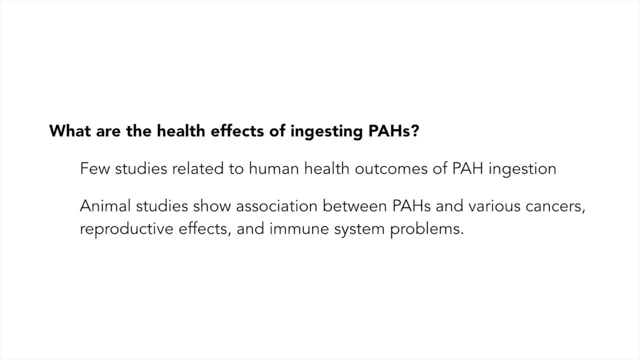 There are only a handful of studies that have shown that lung cancer can cause lung cancer. There are only a handful of studies that have shown that lung cancer can cause lung disease. There are also a handful of studies that looked at human health related to consuming PAHs. 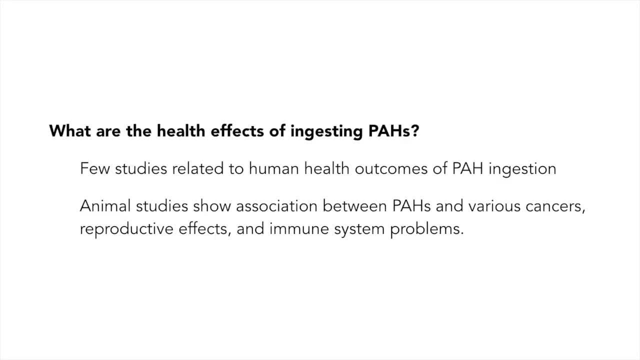 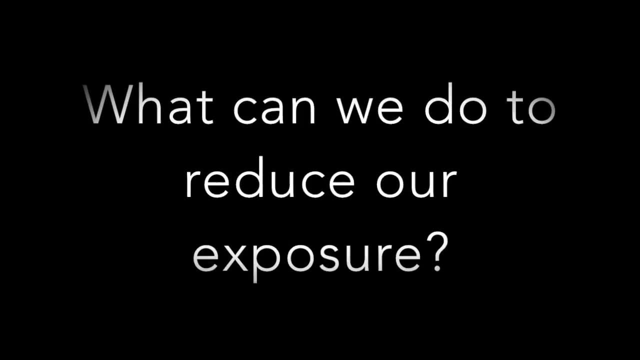 in the diet. However, we know from animal studies that high levels of PAHs in the diet have been associated with several types of cancer, reproductive effects and problems with the immune system. So, finally, how can we reduce our exposure to PAHs? 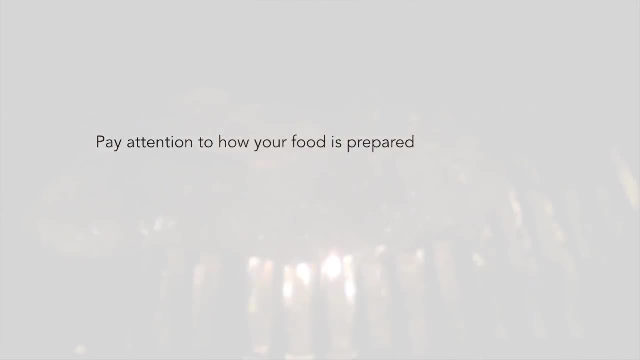 Fortunately, there are some relatively easy things you can do on a personal level to reduce your exposure. Pay close attention to how you cook your meat. If you grill or char boil your food, it doesn't. It doesn't take long or much skill in the kitchen to remove the blackened portions of your meat. 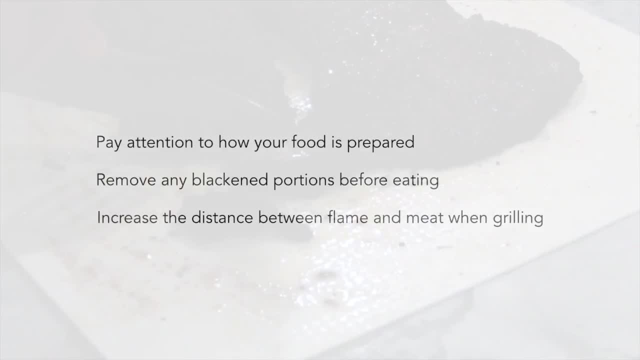 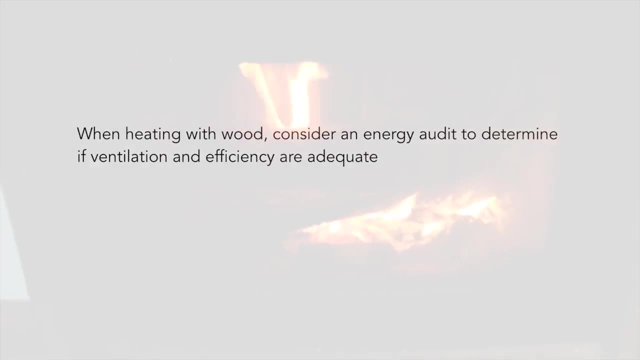 If you can adjust your grill or smoker to increase the distance between your flame and the meat, it may take longer to cook, but it should be less charred. If you heat your home using a wood-fired stove, consider having an energy audit to determine if you have an efficient stove and that it ventilates properly. 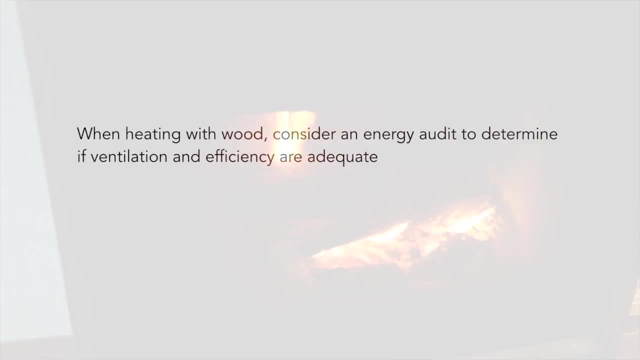 Some cities and counties even offer credits to replace old wood stoves with more efficient models. Eliminating or reducing candles or incense in the home will help with indoor quality as well. If you smoke, there are several options and programs to help you quit. 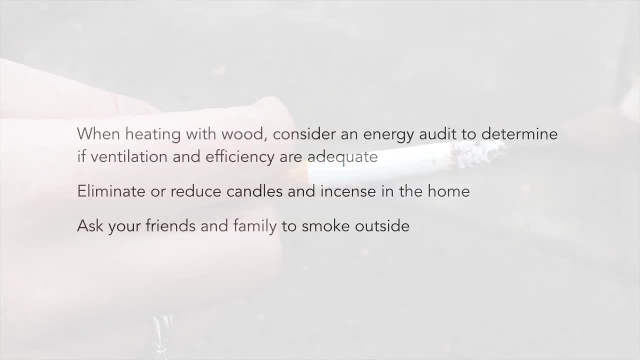 And even if you don't smoke, it's important to keep tobacco smoke outside of the home and cars, particularly if young kids are involved. Ask your smoking friends or family to smoke outside as well. In summary, PEHs are complex chemicals that are produced by both man-made and natural sources. 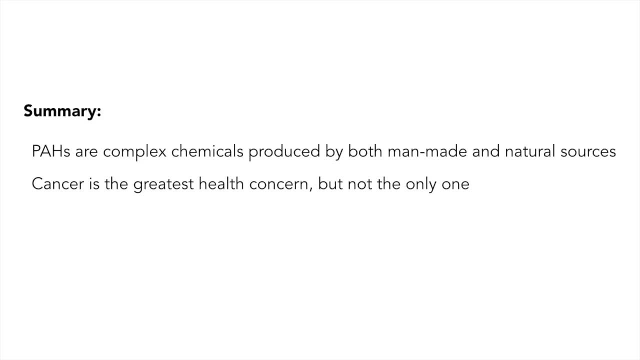 when organic materials are burned. Cancer is the greatest health concern, but not the only one. Smoking, wood heating and grilling or charring meats are our greatest exposures to PEHs. Thankfully, we can take steps to prevent or reduce our exposure to PEHs. 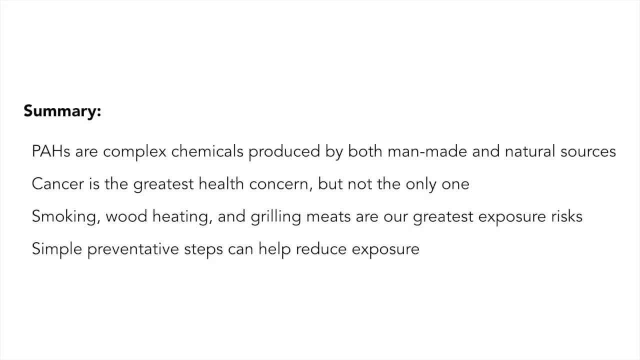 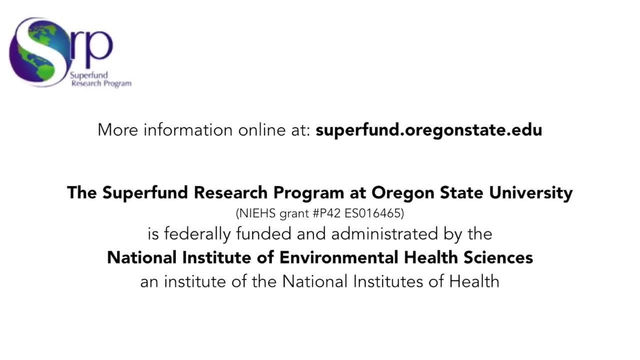 You've already started by learning more about them and why they matter. Again, this is Dr Dave Stone, and thanks for watching our video on PEHs. This video was brought to you by Oregon State University's Superfund Research Program. 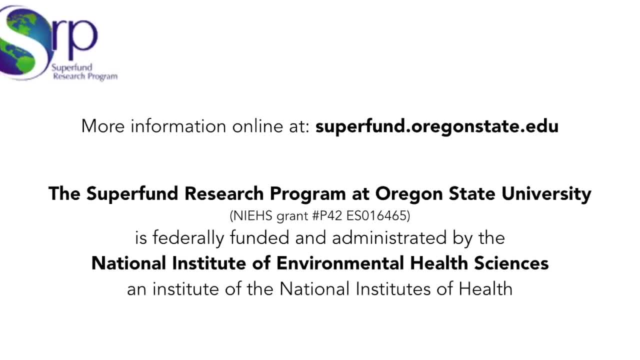 funded by the National Institute of Environmental Health Sciences, grant number P42.. ES 016465..